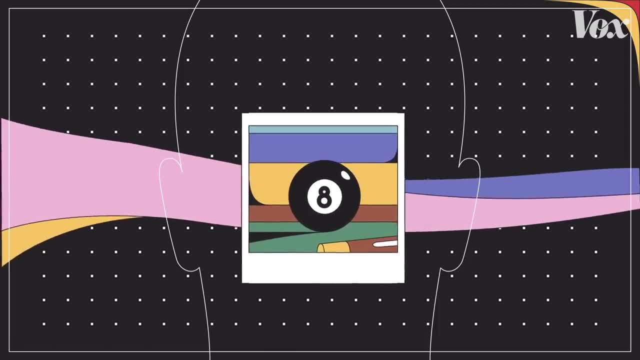 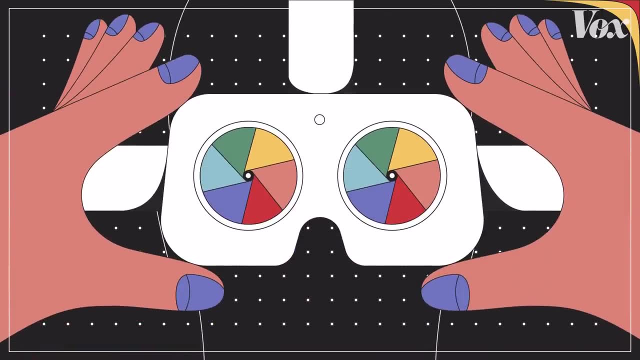 If an object on a screen gets bigger or smaller, or the person on TV moves towards the camera, you don't feel the need to take a step back. But in VR you might want to, because you're not looking at one screen, you're looking 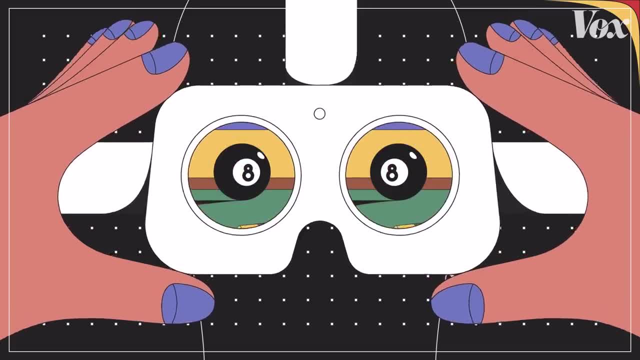 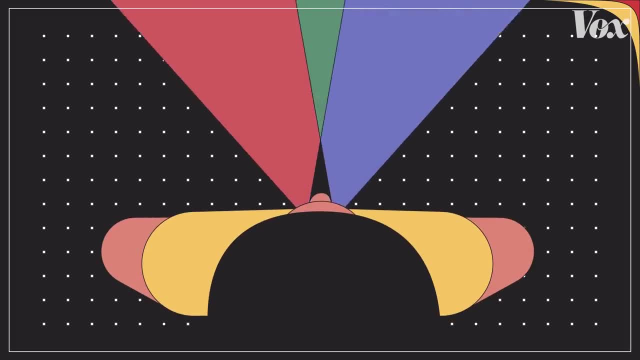 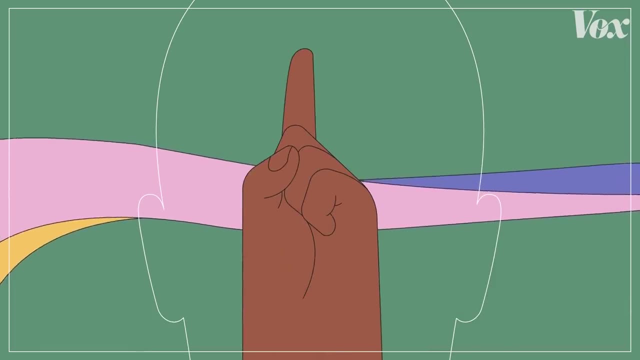 at two, projecting a slightly different image into each eye, Which is how our vision works in the real world. Each eye takes in stimuli from a slightly different vantage point. You can test this: Hold your finger up in front of your face and wink each of your eyes. 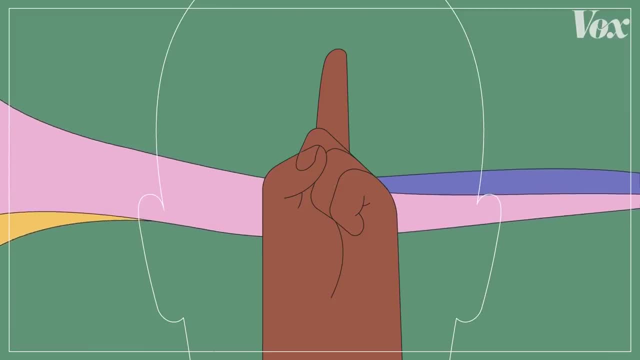 Your finger should jump back and forth. That jump is the difference between what you're looking at and what you're not looking at. It's the difference between what you're looking at and what you're not looking at. It's the difference between what you're looking at and what you're not looking at. 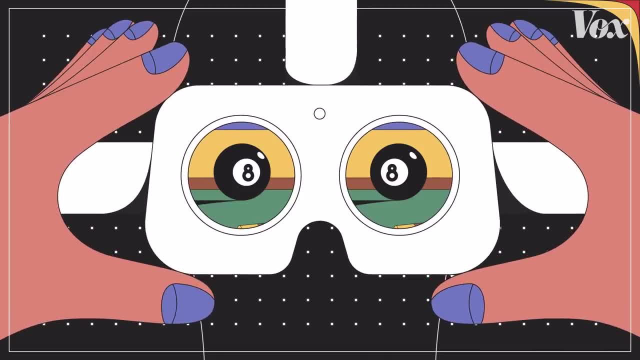 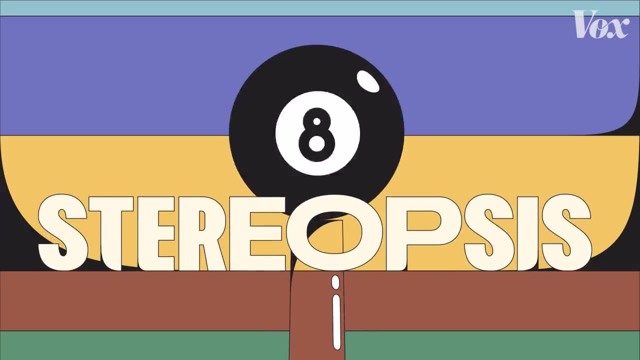 It's the difference between what your left and right eye are seeing, And the difference is between what your eyes see conveys depth. It conveys three dimensions. This is known as stereopsis, and VR developers have spent a lot of time perfecting it. 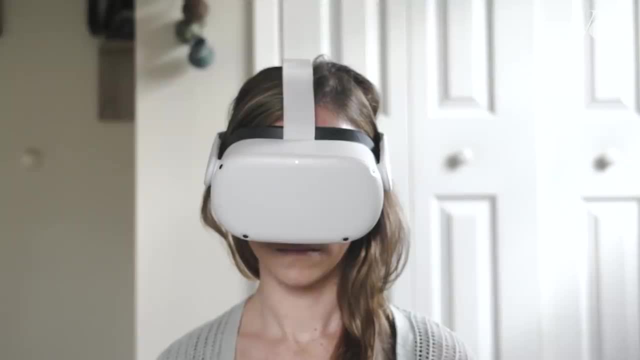 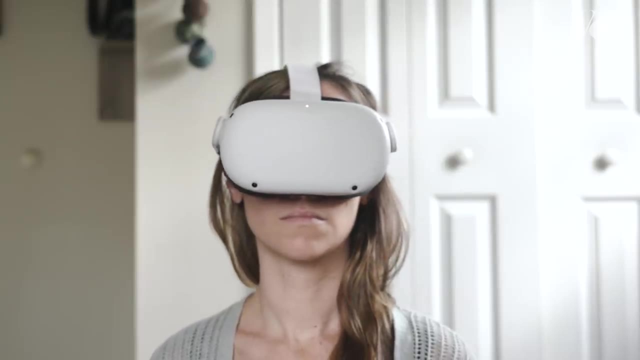 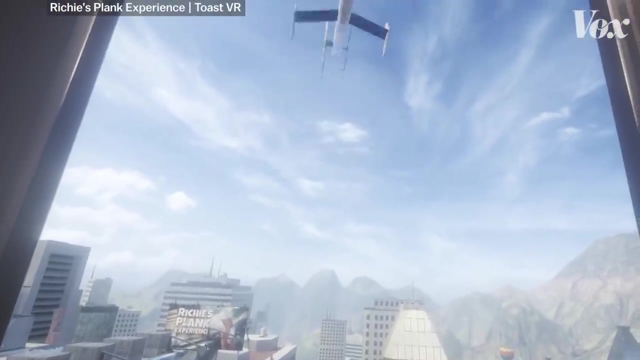 But what use is depth if you can't move through it? Which brings us to the next most important way. virtual reality tricks your brain. You are the camera and it's fast enough where your brain starts interpreting it as your perspective. Speed tracking allows a person in VR to look and move around a fake world in the same. 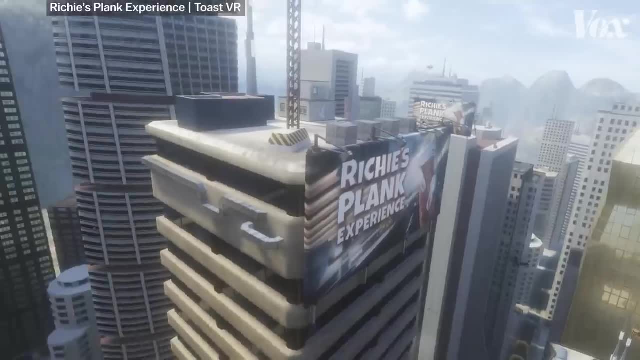 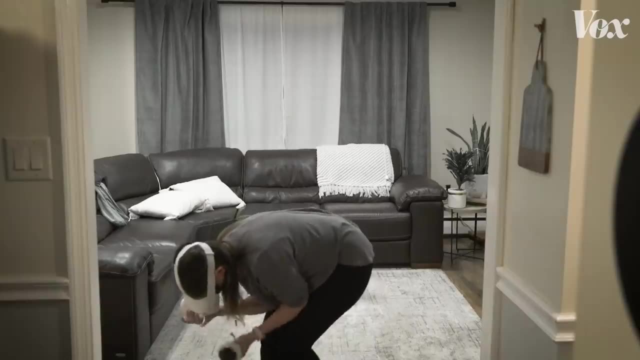 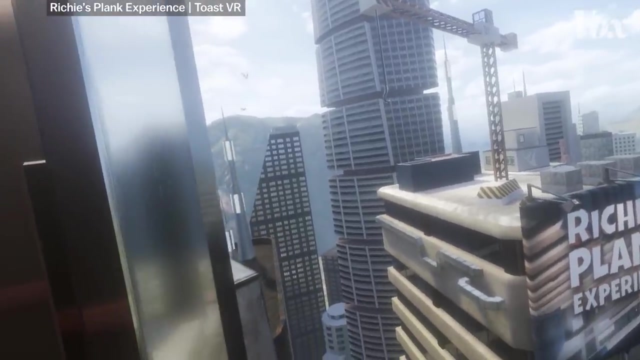 way that we look and move around, a real one. If you look to the left, you'll see more of the world to your left, And if you look down- Okay, maybe don't look down. Other subtle effects make virtual spaces feel more real, like 360 audio, which is a big 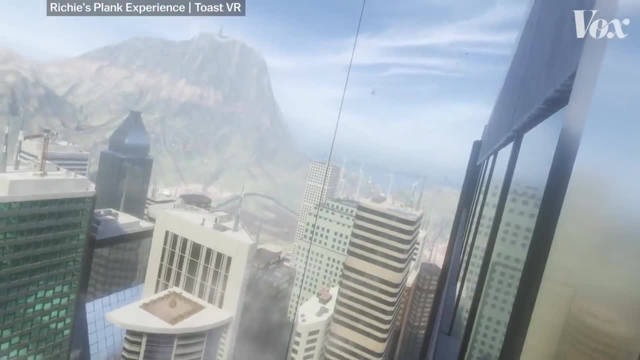 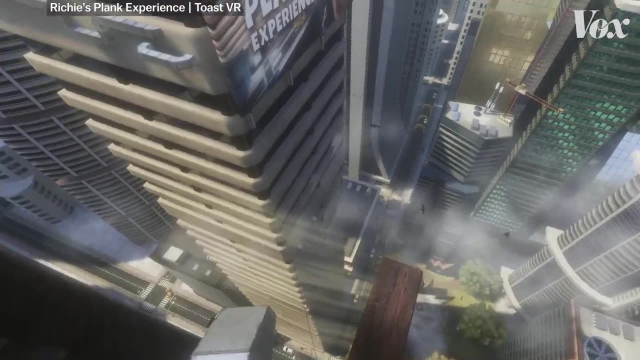 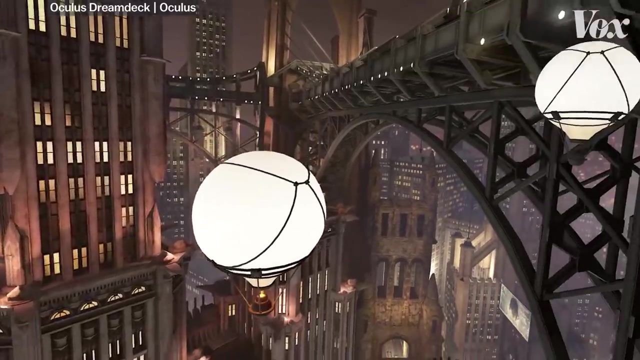 part of the plank experience. As you turn your head, the wind will subtly change, The plank creaks And if you listen closely, The heartbeat slowly begins to speed up. Our brain takes all this new virtual stimuli and begins to believe this is reality. 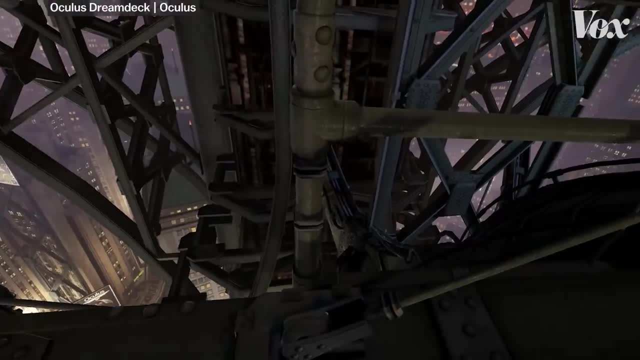 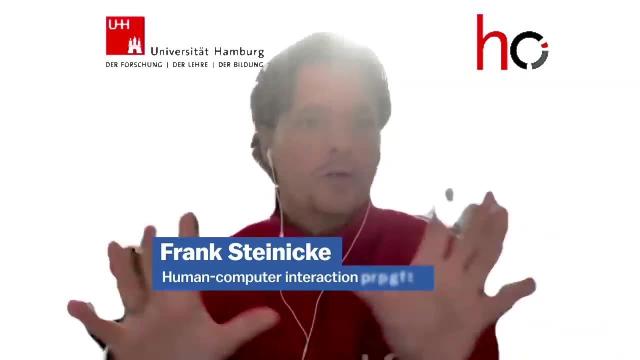 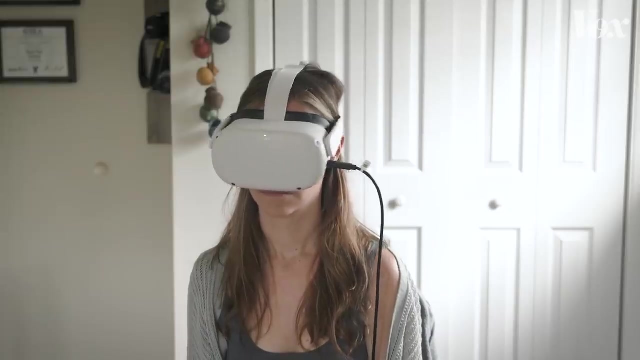 Our brain has never really learned within the last 150,000 years to actually distinguish between computer-generated content and the real world. Dr Frank Steinecke has been studying immersive technologies like VR for nearly 20 years, And if all the cues that we perceive in the virtual environment are so similar to the 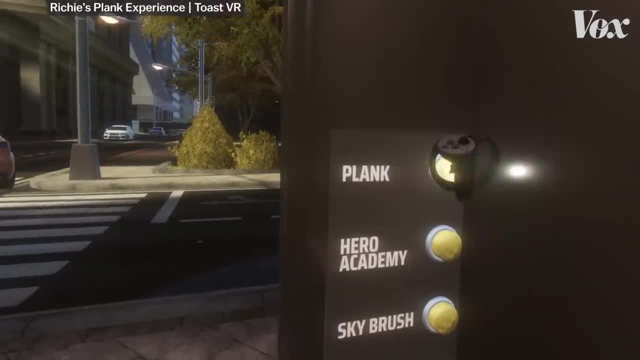 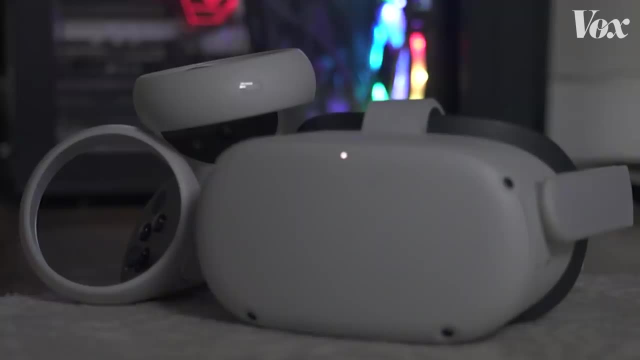 cues that we get in the real world. It makes kinds of sense that we are unable to clearly distinguish between both. Our brains quickly adapt to virtual environments, largely because it's wired to trust our sense of sight. There's some research showing that approximately 80% of all the information that we perceive 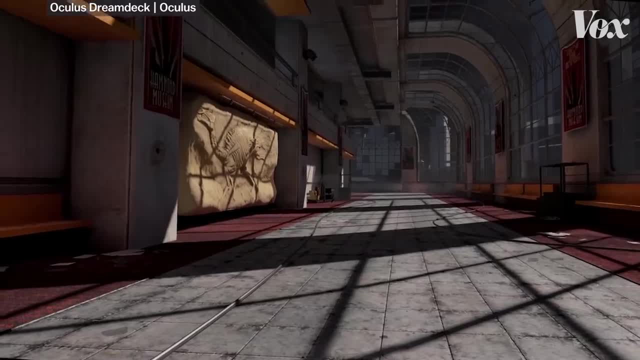 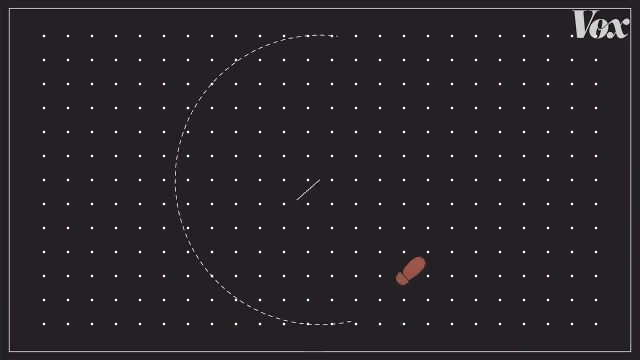 from our environment are based on vision, And this allows VR developers to manipulate our reality even further. We found out about 10 years ago is that we, if we guide users on a circular arc with a radius of 20 meters, they have no chance to identify that they actually walk on a circular. 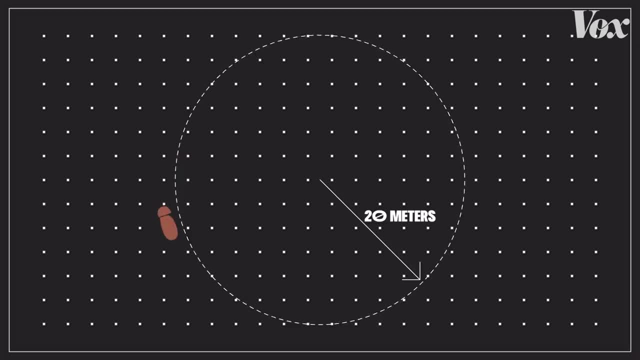 arc with a radius of 20 meters. They have no chance to identify that they actually walk on a circular arc with a radius of 20 meters. They have no chance to identify that they actually walk on a circular arc with a radius of 20 meters. 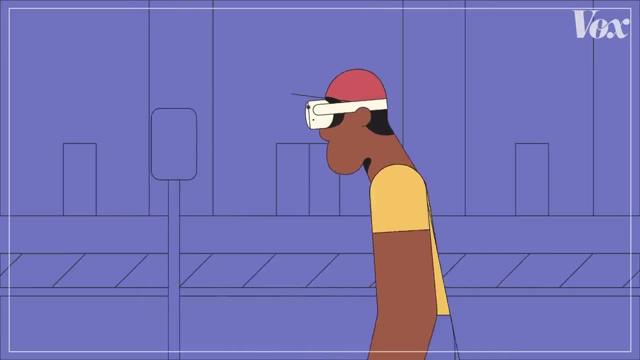 They have no chance to identify that they actually walk on a circular arc with a radius of 20 meters. But they can walk on a circular arc with a radius of 20 meters. They can walk on a circular arc with a radius of 20 meters. 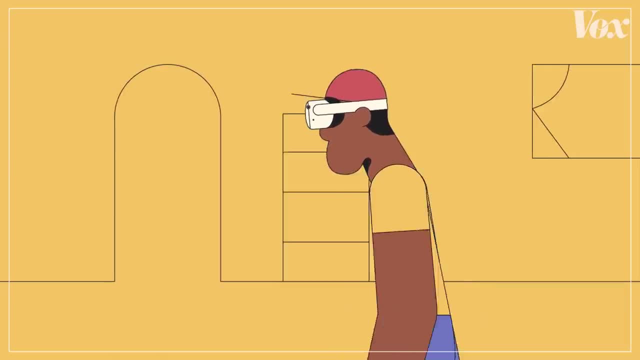 They can walk in a circle in the real world when they see a straight path. in the virtual environment, You can walk an entire virtual city without ever leaving a room. Once we believe the environment is real and accept that we're actually in it, our brains. 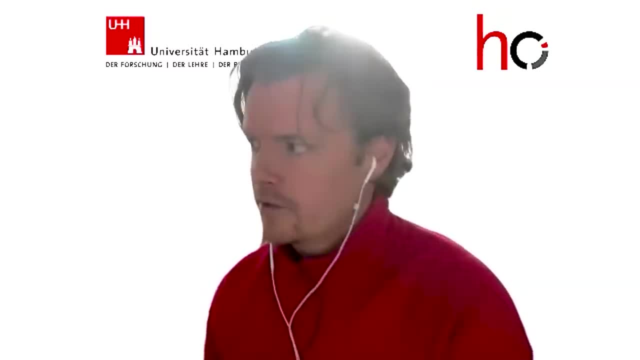 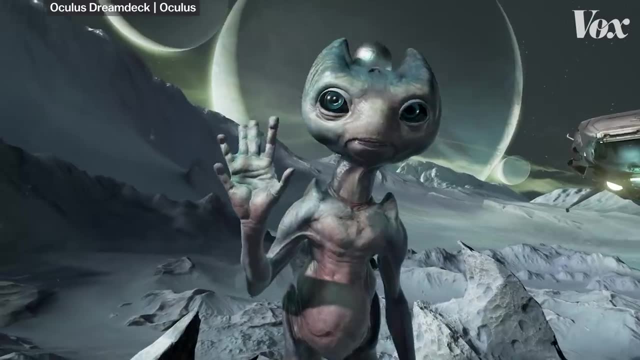 then go on to fill in some other blanks. There are interesting findings that, for example, if you are in the virtual world in a very, let's say, snow or icy environment, people feel cold, Although they're in the real world, maybe in a hot environment. 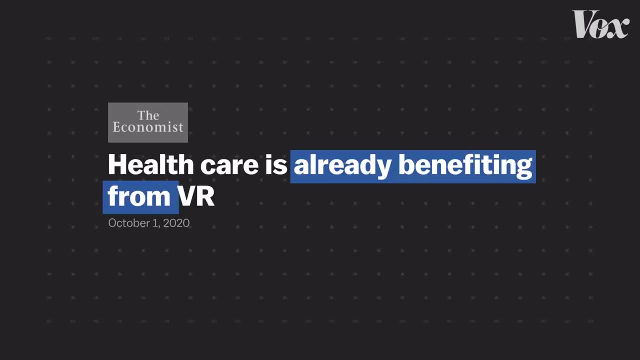 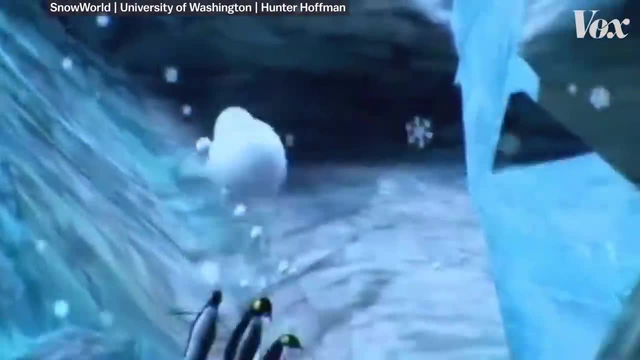 I feel cold. I feel cold actually shown a lot of promise in the medical world, from reducing pain and burn victims by immersing them in a snowy world while their bandages are being changed, and with exposure therapy that helps people with phobias like a fear of heights and body dysmorphia. 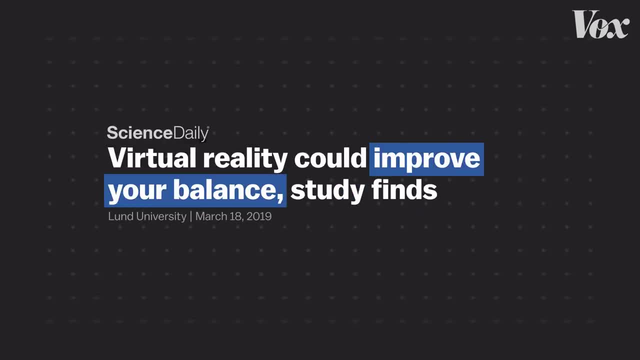 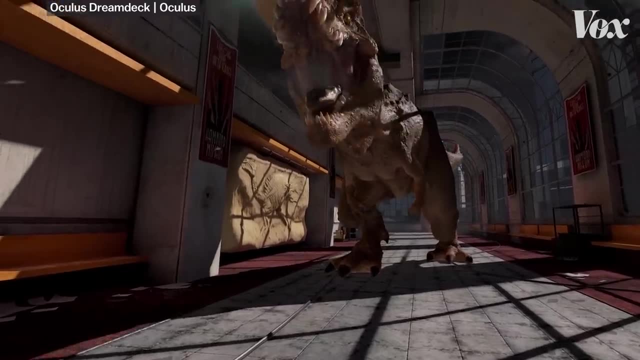 It's also being used for physical therapy, like assisting elderly people with their balance. Right now, we're still tethered to a system with a headset on our faces. The graphics are nice but not perfect, and so we're not fully immersed when we hover. 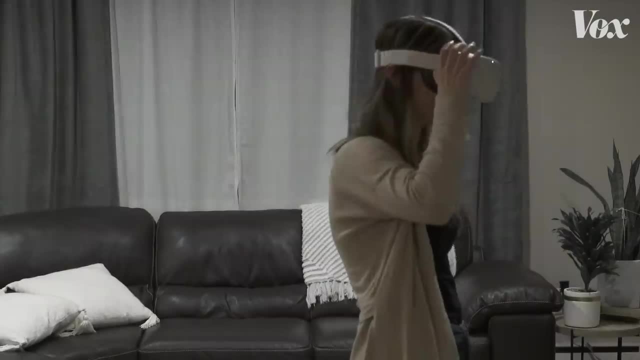 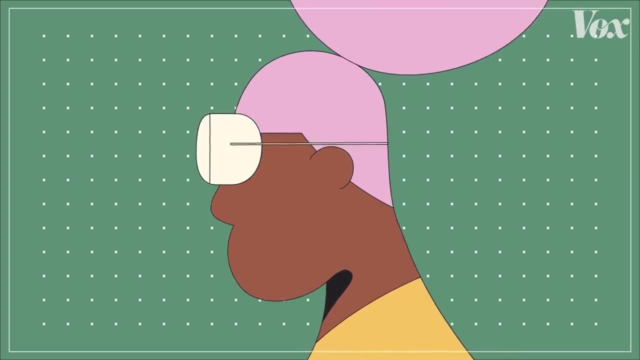 80 stories above the ground, That is, we can still remember to take the headset off. Steinecke cautions that it might not always be that way. We can easily assume that within the next five to ten years or so we will not be able. 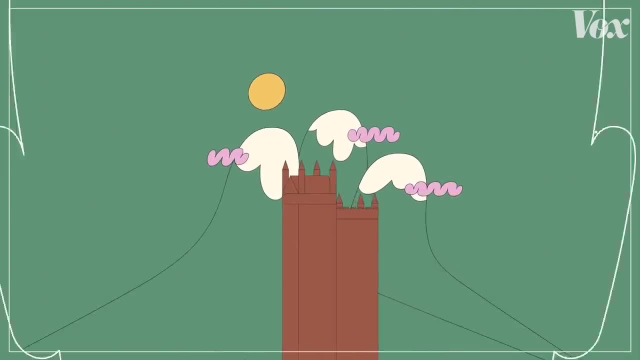 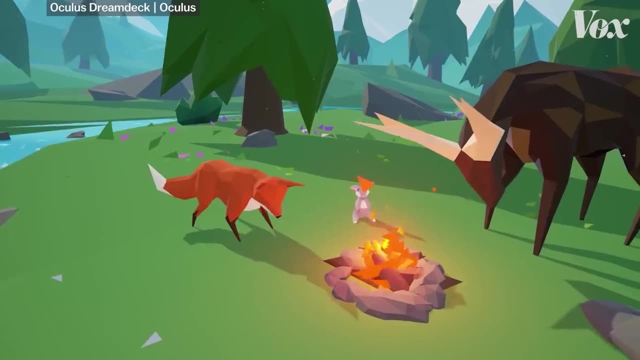 to distinguish visually computer-generated content from real-world content anymore. And then, of course, there are a lot of ethical questions. For now, VR might not look exactly like reality, but it follows a lot of the rules our brain has learned to perceive as real. 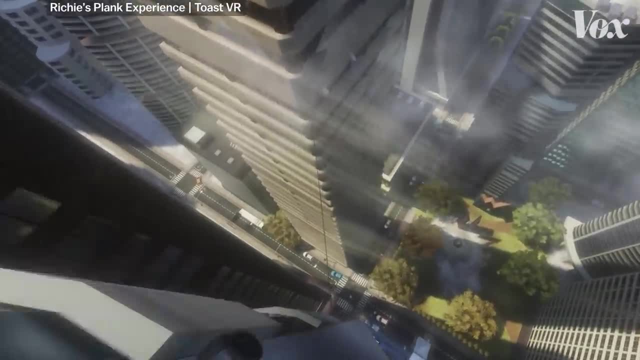 And that's often enough to make us sweat. Thanks for watching and I'll see you in the next video. Bye.